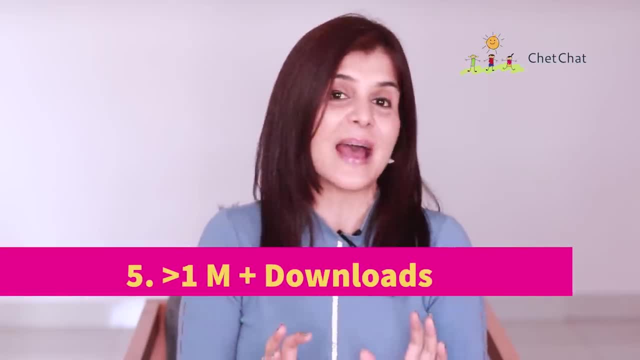 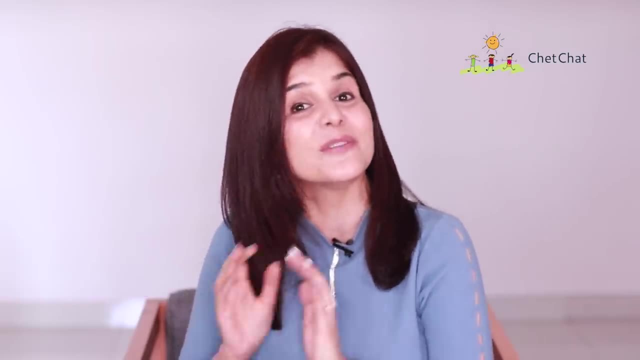 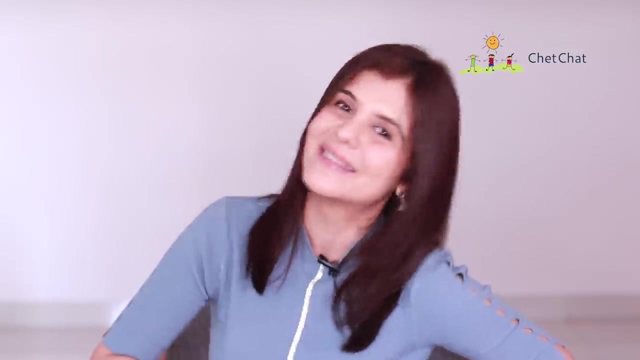 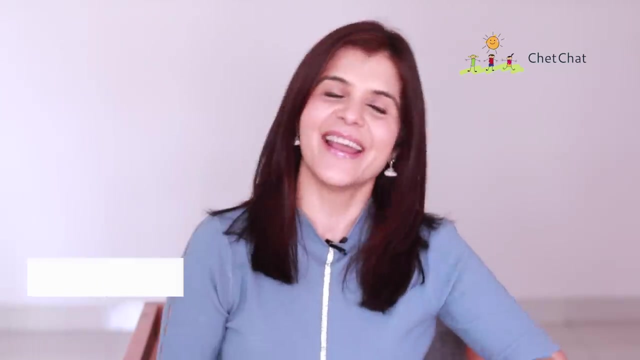 and made sure that users love these apps. apps featured on our list also have a minimum 1 million download. in fact, some of these apps also have up to 10 million downloads. now i promise that you're going to love these apps, and number six will surprise you, so let's get going. hey, this is chetna and you're watching chet chat and this. 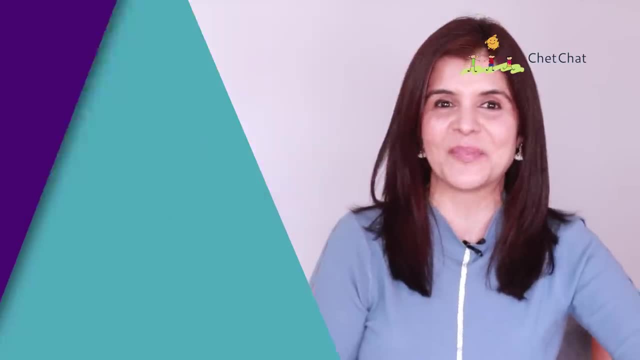 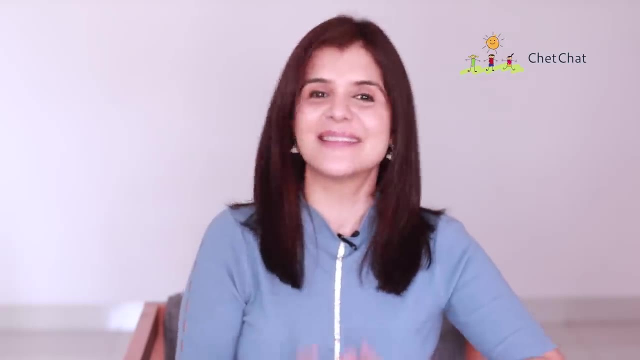 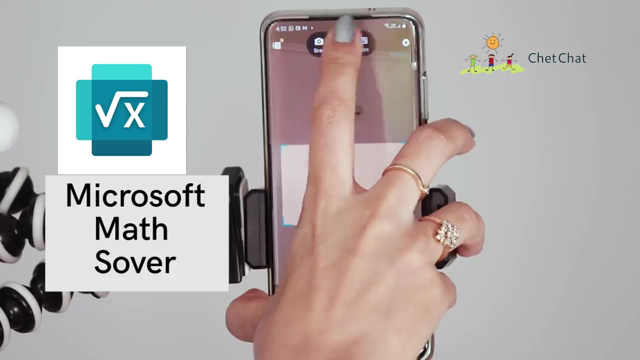 is my list of the top 10 free study apps for you. at number one we have an app straight from microsoft called microsoft math solver. this is the perfect math app, and you get three options here. you can either scan your question out or you can draw something. so let's say you write. 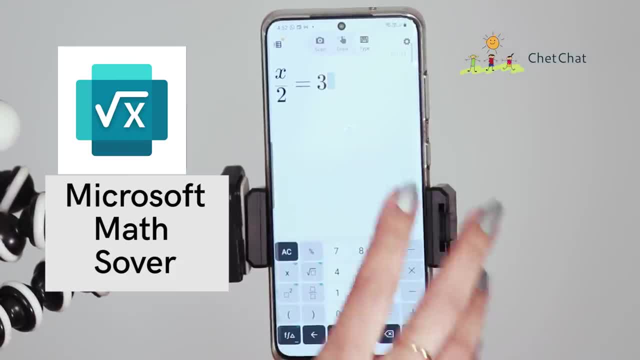 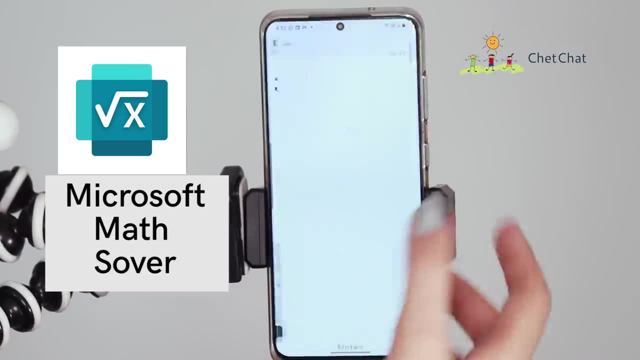 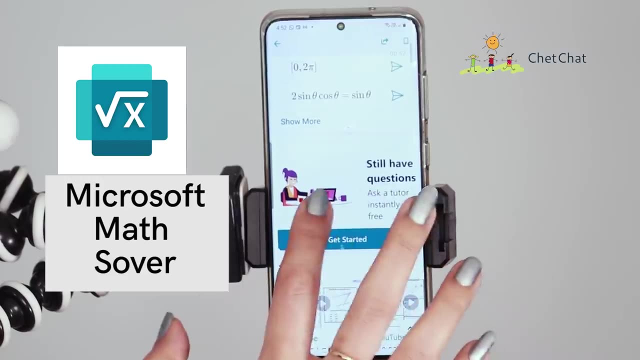 or you can type out your question and they have a little bit of a scientific calculator here and if i tap here, look at the kind of topics they have and let's say you want to go here, you'll have some questions. those questions will have graphs and in the beta version you can even get a 20 to 30 minute free tutoring class. the app has more. 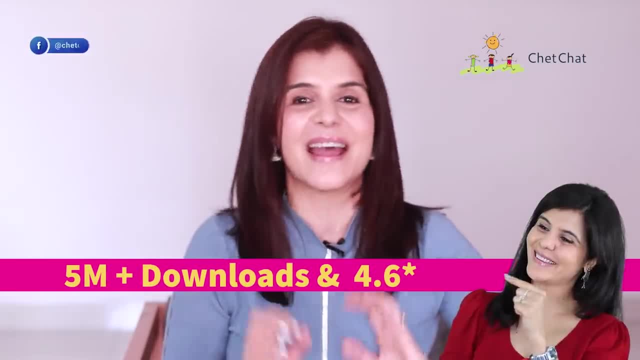 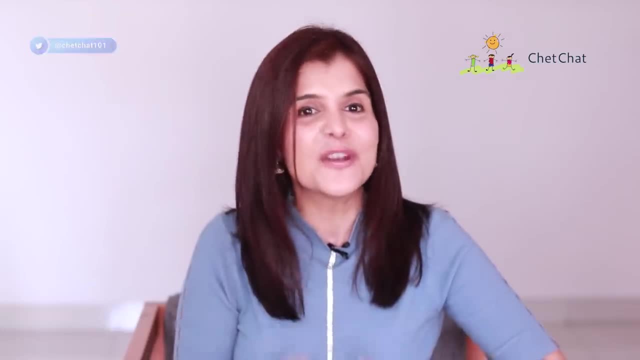 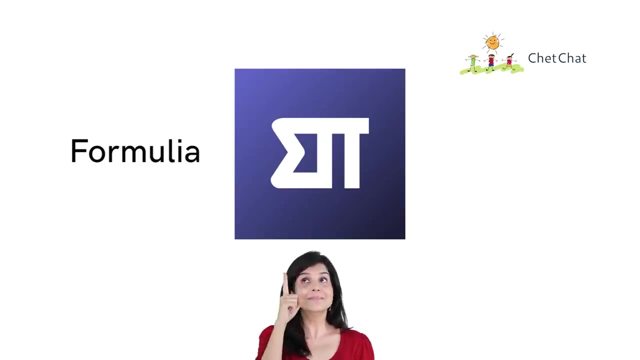 than 5 million downloads and is rated at an average of 4.6 on the play store. the app is not only 100 free, but also free from all ads, so no problem if you have a math problem. at number two, we have a very interesting app called for molia. it's a very cool. 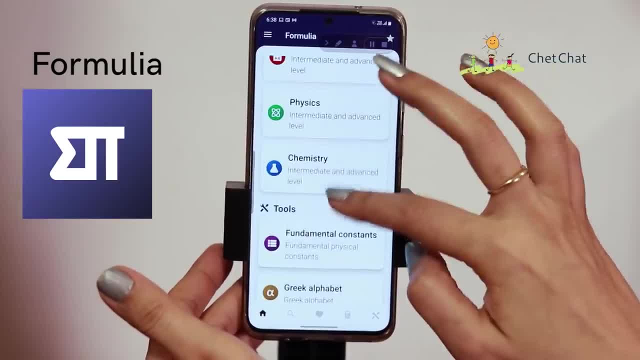 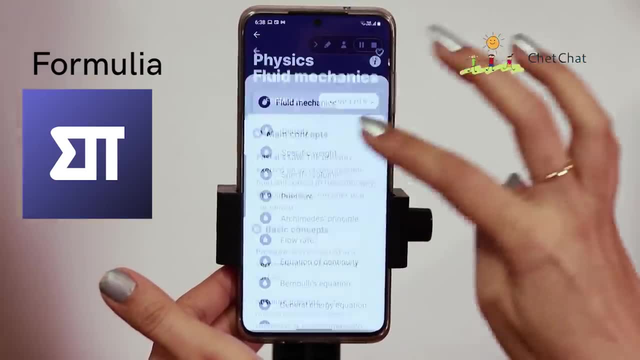 app. it gives you all the formulae of, let's say, math, physics, chemistry. let's click on physics. these are the kind of topics you get. let's see. you'll get formulae. you'll get all the concepts here. as you go down, you'll get some fun days on the periodic table. what's interesting is, with the 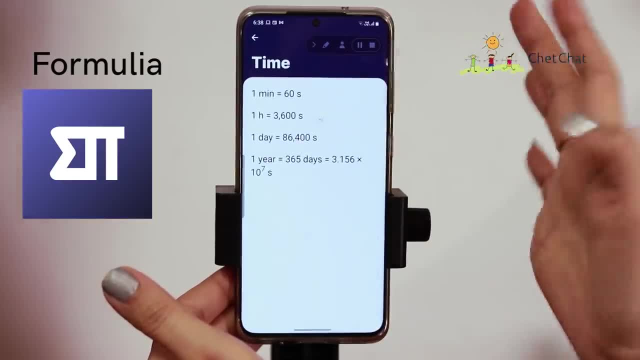 tools here. you can get unit conversions, for example. you want different conversions from one unit to another. you can also use different conversions and our softwareال say: let's say this computer salary Millionaire, finishing the fifth place in math, math, las Una lava. you can get different conversions, for example, you want different conversions from one unit to another. you 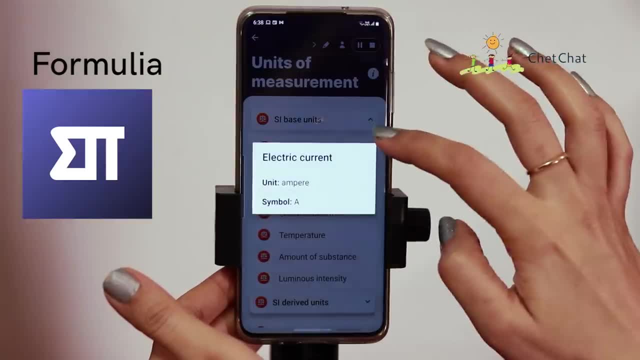 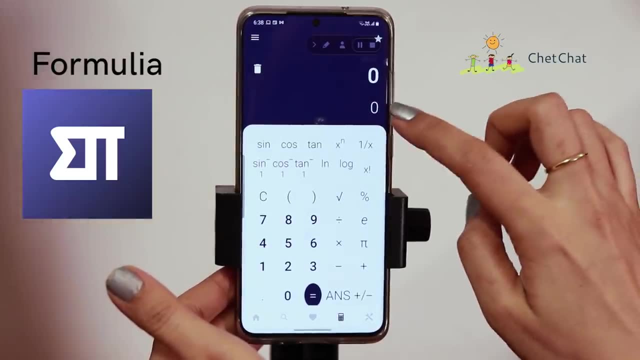 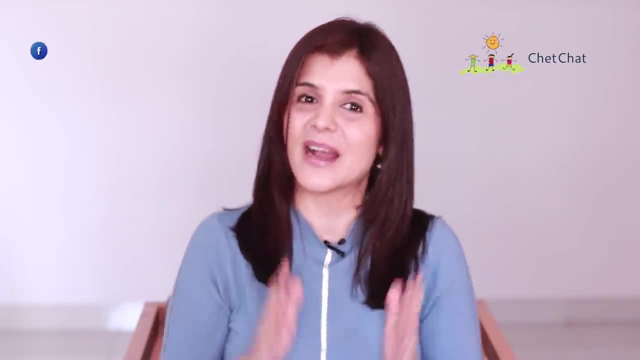 so get maybe what are the different units of electric current, etc. what i really love about this app is this scientific calculator which you get on the go. the app has more than 500 000 downloads and has an average rating of 4.7. a compact and useful app for all students. if you're. 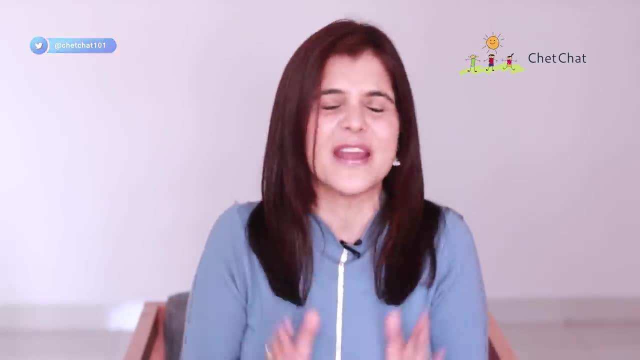 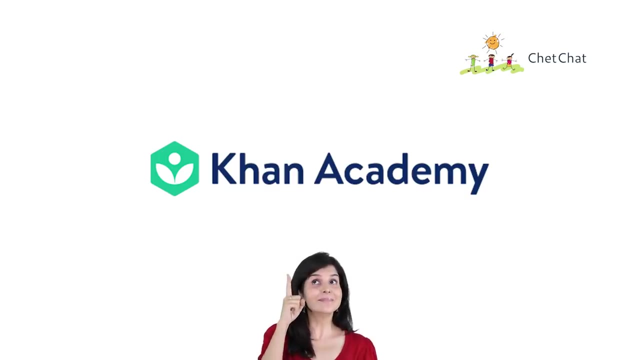 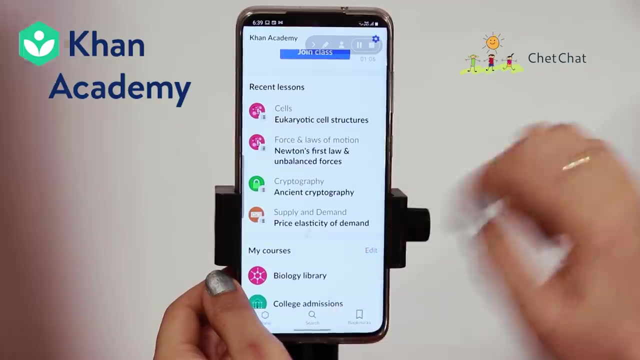 using any of these apps or any other free apps that you find very, very useful, then share that with us in the comment section. at number three, we have our all-time favorite: the khan academy. khan academy is a very popular app providing world-class content on school education for the 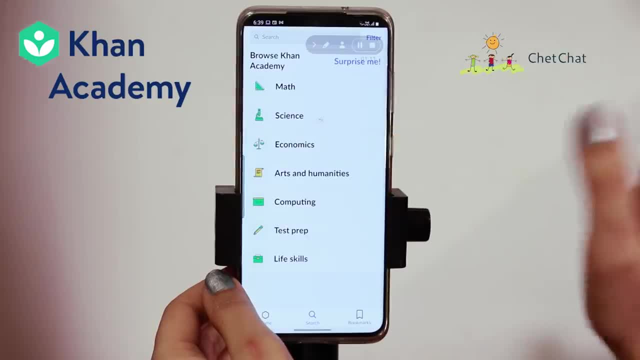 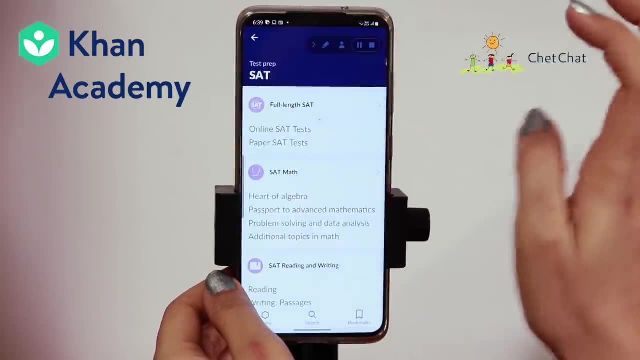 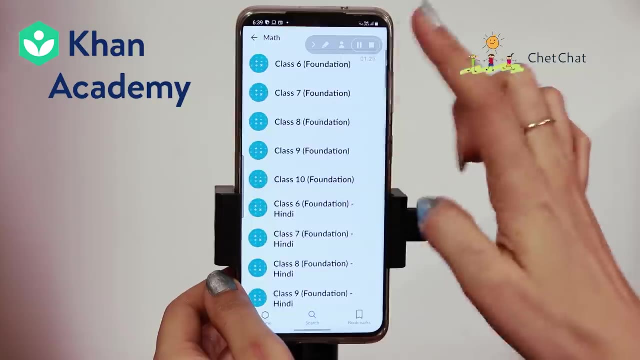 longest time with the same amazing quality, all for free. so for example, to test prep: very interesting. if you're preparing for, let's say, the lsat or the sat, you're going to get a host of material here, including tests and mock tests etc. so let's say we click on math. look at the range of math that you get, different topics, you click. 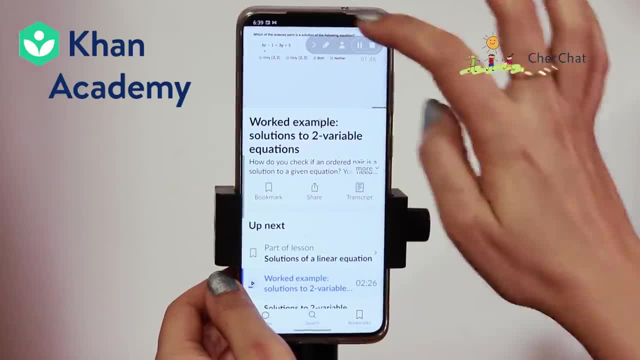 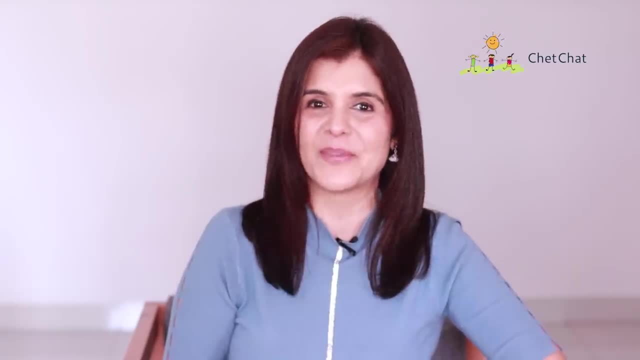 which of the ordered pairs is a solution of the following equation? they have more than 10 million downloads in the play store and have an average rating of 4.4. at number four, we have an english app called bbc learning english. the app has more than 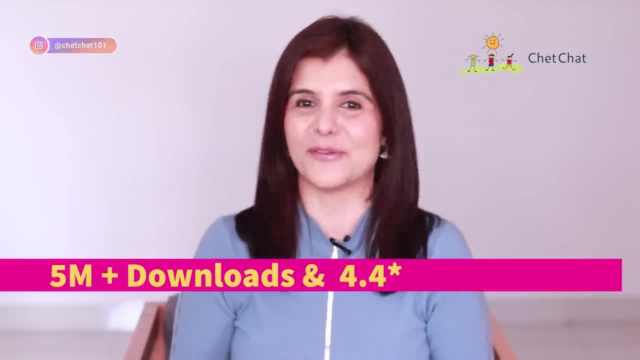 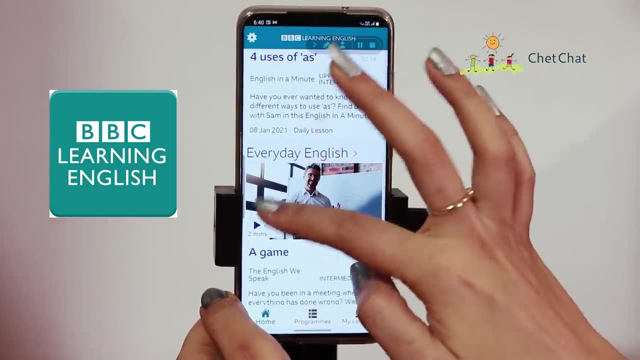 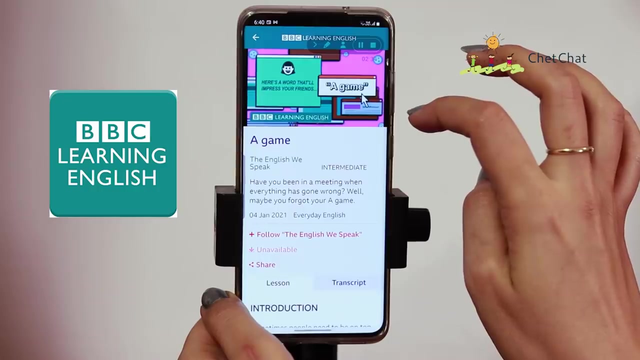 5 million downloads and an average rating of 4.4. the app is super catchy and fun to learn. you'll get a lesson for the day and as you go down, you could even click on one of these videos. hello and welcome to the english we speak. i'm feifei and i'm roy. what i love is when you go. 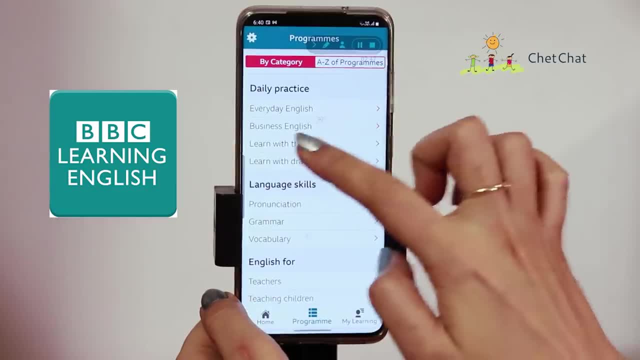 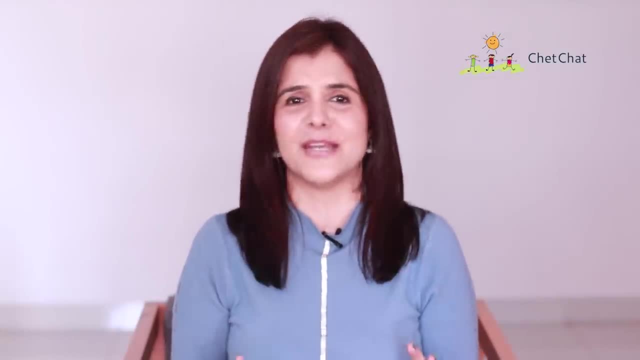 under programs, you get the whole list. you want business english, you want to learn with news, you want pronunciation, grammar, vocabulary. the best thing is that you don't have to pay a penny for it. so mesmerize the world with your english skills. and if you're looking for apps that can help you, 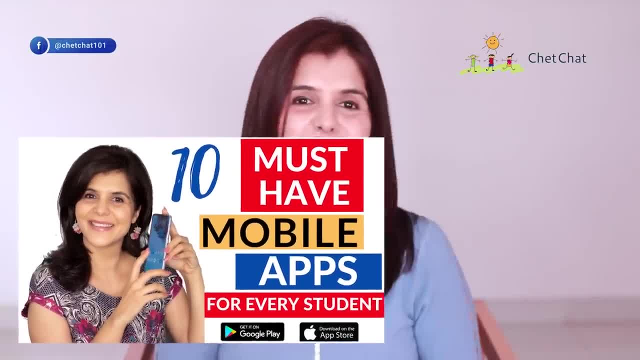 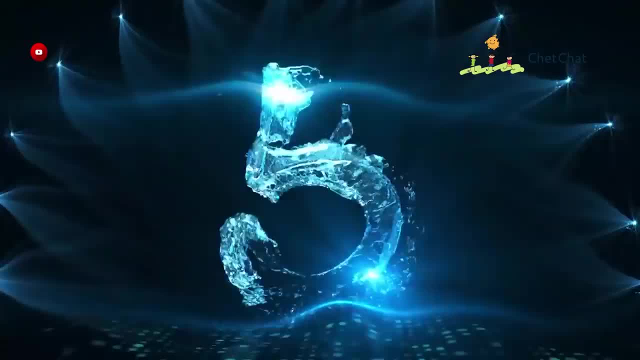 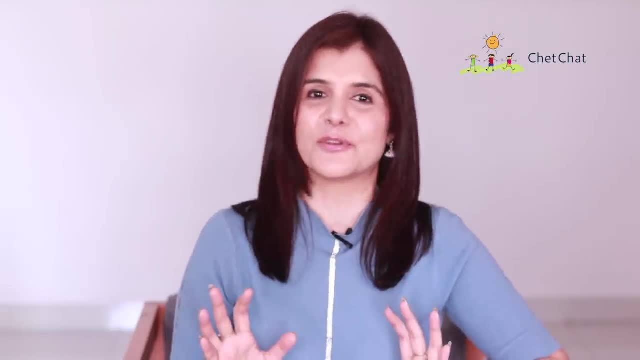 with more than just studying. then do watch our video called top 10 free apps that every student should use and i will drop a link for you in the description box below. at number five is mimo. mimo is a perfect partner for learning various computer languages. 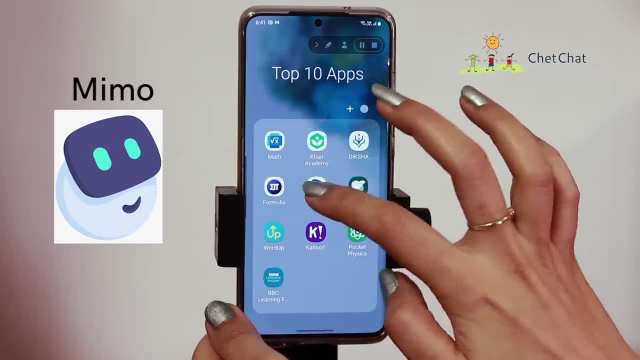 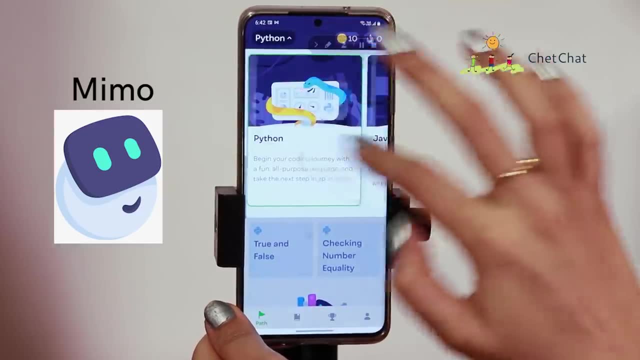 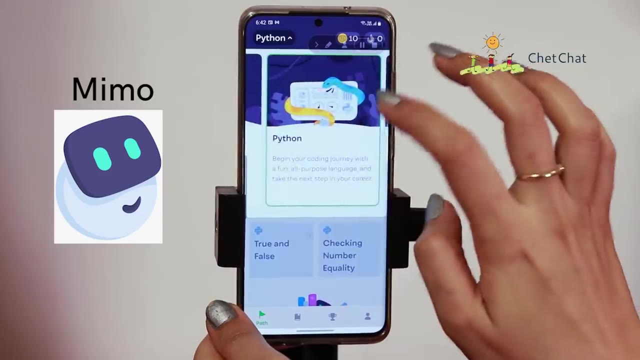 for basic and intermediate levels, and if you have no prior knowledge of any coding, that is no problem. for mimo, you've got an option here when you click on this. here are your options. you want to do web development? you want to learn python, javascript, html and css? let's click on python. it's a bit like a game. you can see some featured. 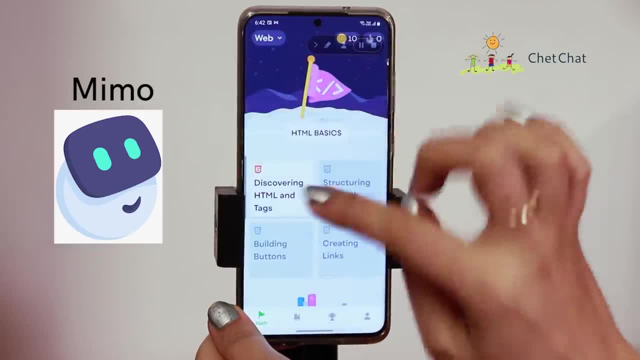 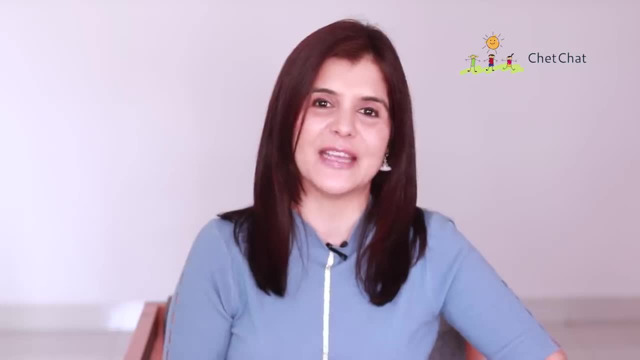 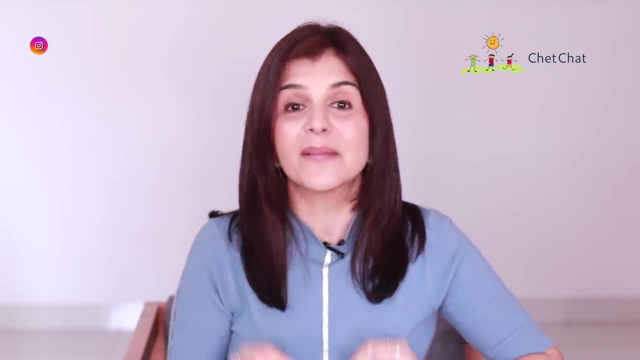 projects, maybe some challenges, ton of stuff. but you've got to build. you do one level, you go to the next. that's how this app is structured. the app is completely free, with 4.7 average rating and more than 5 million downloads. the best thing about the mimo app is that at the end you get a personalized 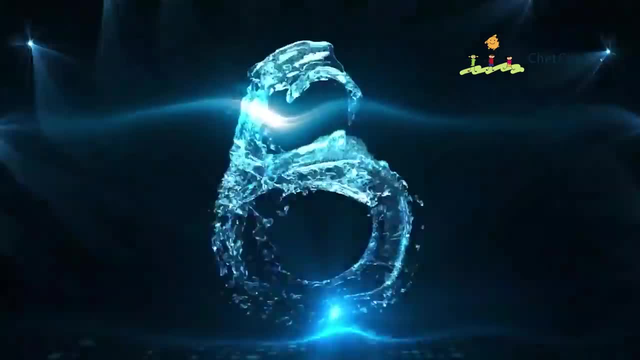 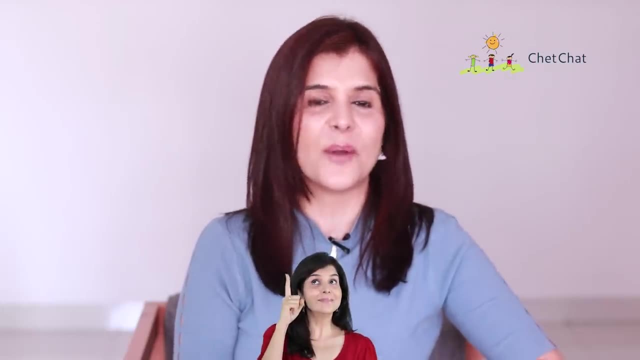 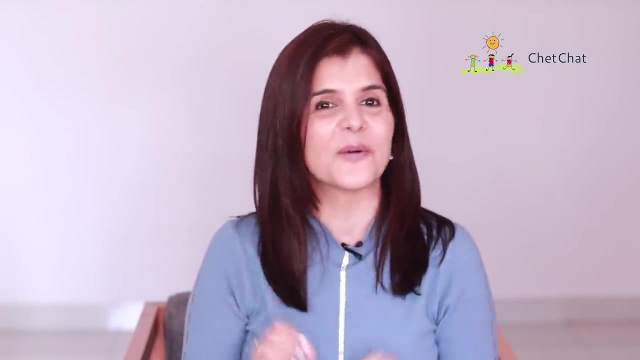 certificate as well, so keep coding and creating. at number six, we have a testing app called class sati. class sati is a relatively new app with 100 000 downloads, but their commitment to provide valuable content made it to our list. they score a 4.5 on an average rating on the play store. 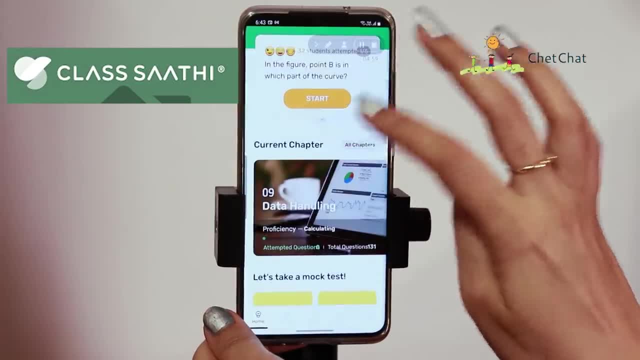 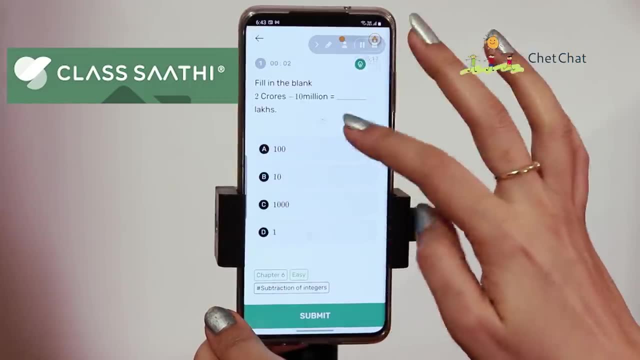 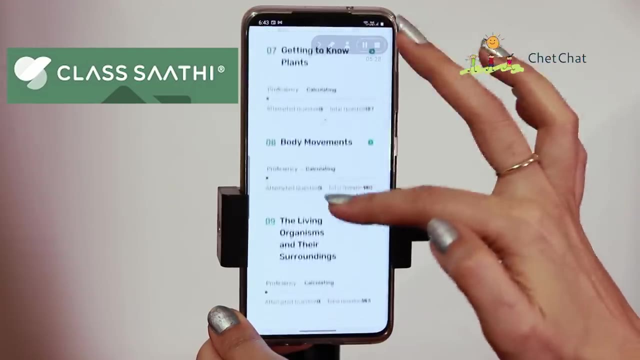 Sathi helps students from class 6 to 10 to take mock tests in math and science. so let's say I pick integers and then I start getting questions. let's say you want to go into science and you've got all your chapters and you can have a whole host of questions to practice from. 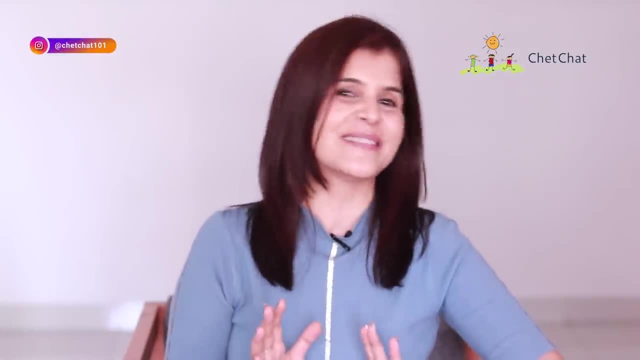 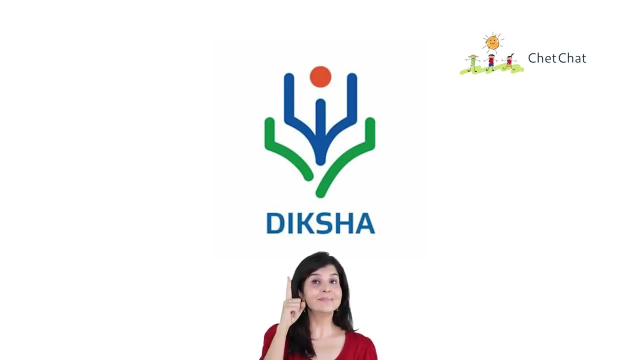 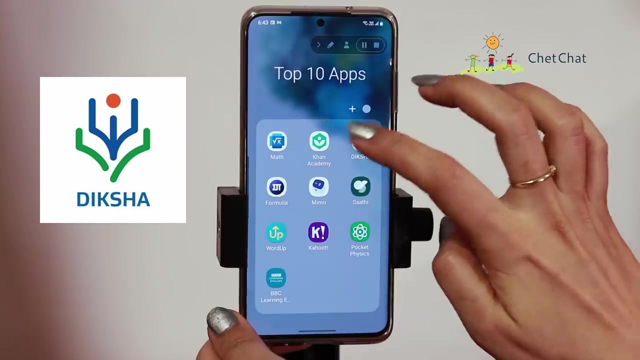 successful completion of required tests can also get you a certificate. so practice more and learn more. at number seven, we have a study app from the ministry of education government of india called diksha. diksha provides one of the most diverse and elaborate resources for school education, ranging from class 1 to class 12.. is english medium, you get different. 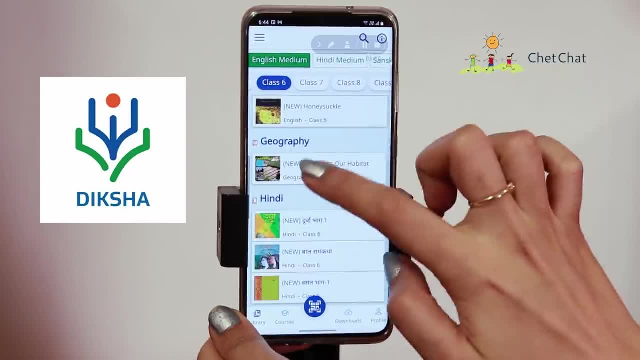 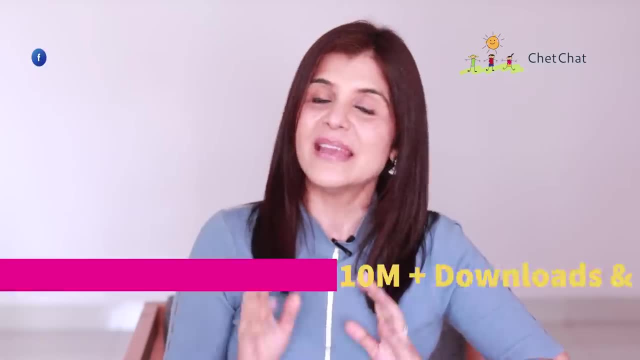 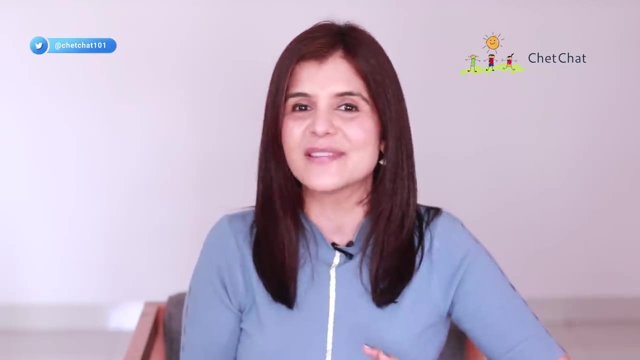 languages that you can pick from here and as you go down. let's say you choose geography- you've got an option of either choosing all the video resources or the documents. the app has over 10 million downloads with a 4.4 average rating, so a 24: 7 library is waiting on your. 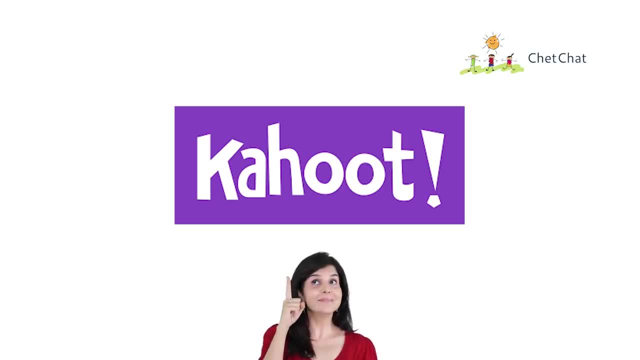 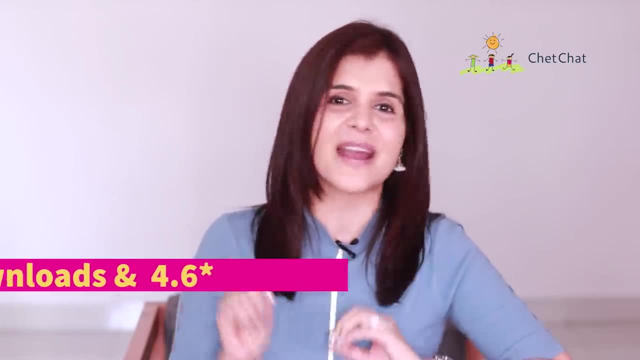 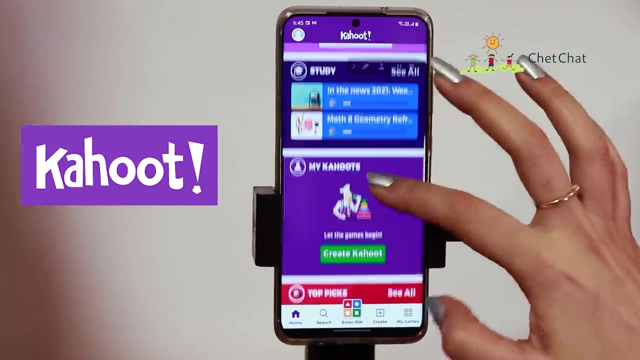 device. at number eight, we have a quiz app called kahoot. kahoot has a 4.6 overall rating and more than 10 million downloads. in fact, kudos to the team of kahoot, who've created this super engaging and helpful app for students. what you're going to get is the ability to play with your friends, so if 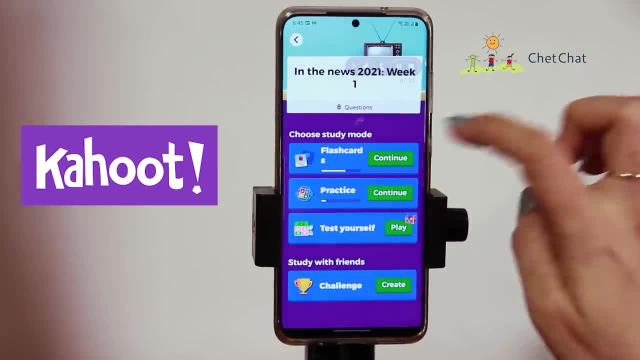 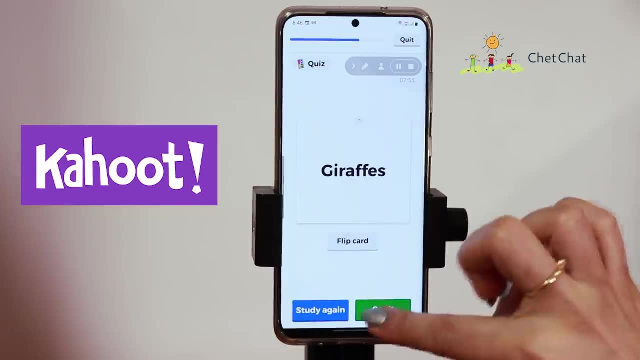 and let's say i pick in the news 2021, i can either study or i can play, and then they're going to keep putting flash cards in front of me. you flip it and then you say, got it. it's pretty cute, it's much like a game. so what are we waiting for? 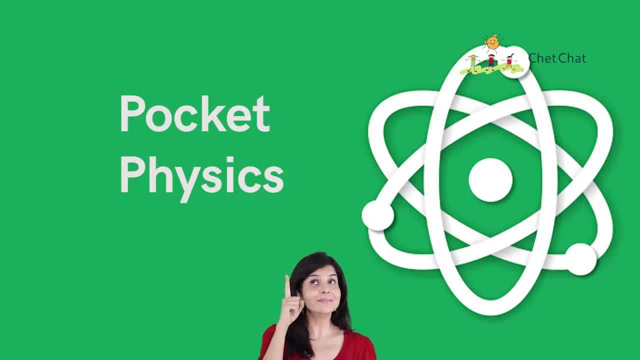 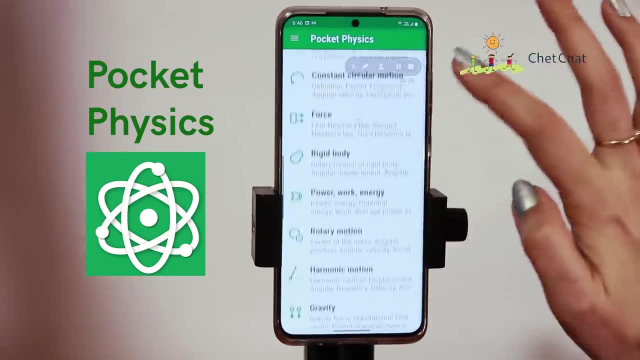 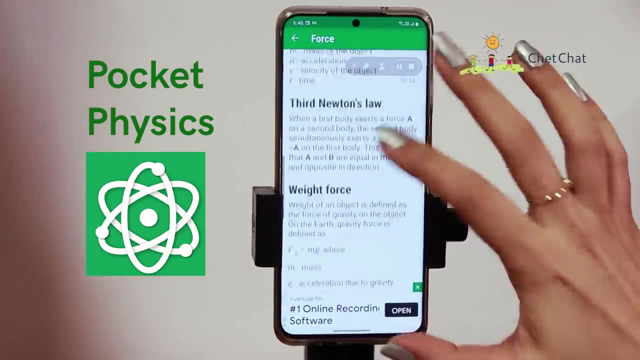 let's quiz at number nine. we have a physics app called pocket physics. in fact, true to its name, it's handy and a simple app for physics concept. here's your list of topics that you have. you click on one of them and it's going to tell you about the concepts, the main concepts, the formulae. 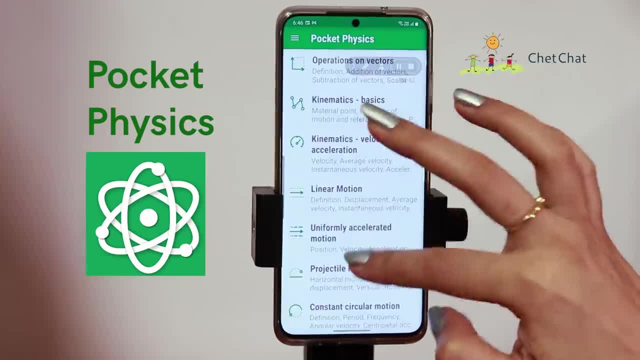 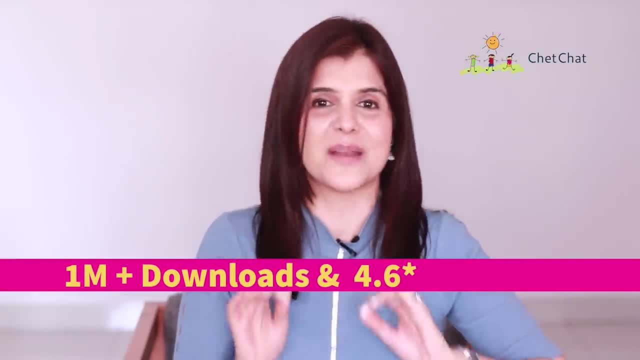 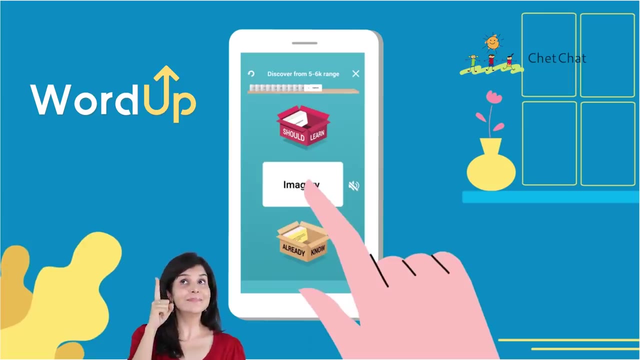 sometimes the derivation of the formulae and a few graphs: physics in your pocket, easy peasy. this app has more than 1 million downloads and an average rating of 4.6, and at number 10 we have word up. word up is one of the most advanced ways of learning vocabulary, and no wonder. 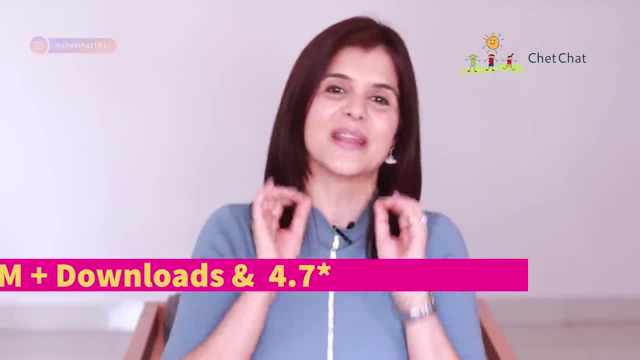 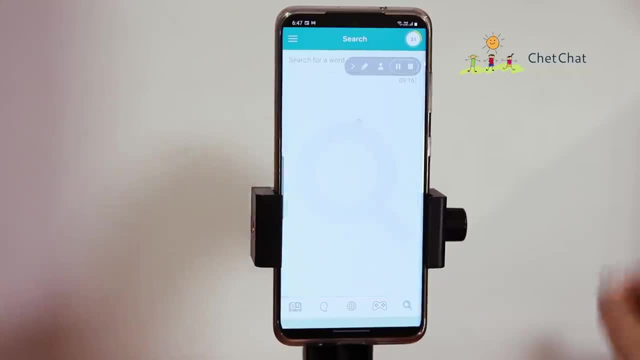 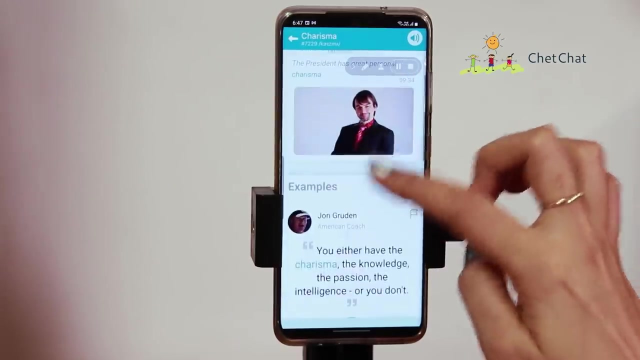 they have an average rating of 4.7 and more than a million downloads. so when you open the app, they give you a set of like a quiz. but what i like is this: magnifying lens- and let's search for a word here- so once i click on it, they show me the definition, maybe an image, some quotation and 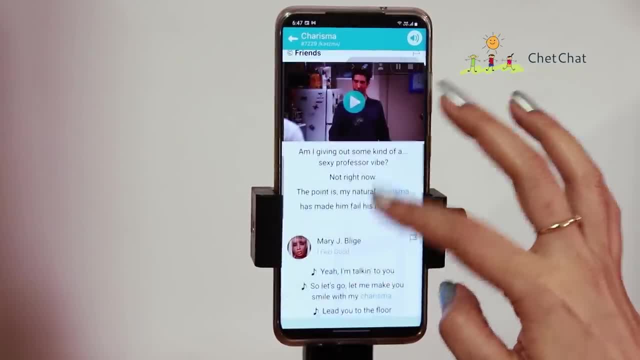 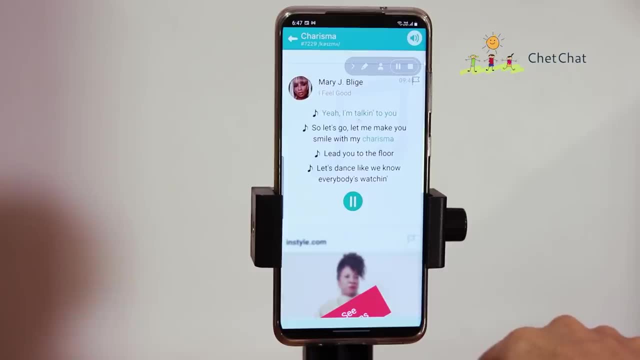 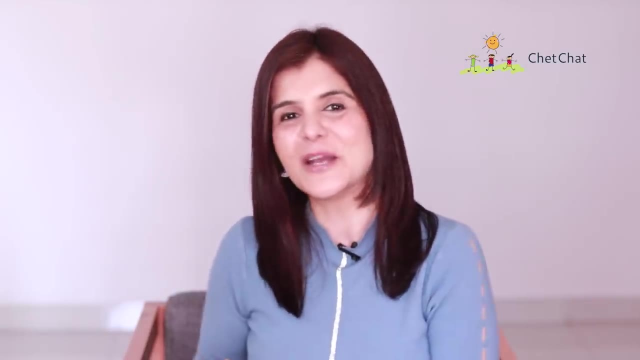 they also give. give me a little video from maybe a popular show and some poem that i want to listen to. yeah, i'm talking to you, so let's end the forever search of a perfect dictionary in your pocket with word app and if you've enjoyed this video. 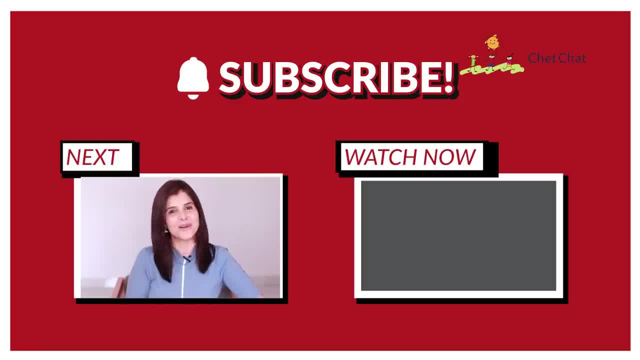 share it with your friends and see you in the next one. happy watching.